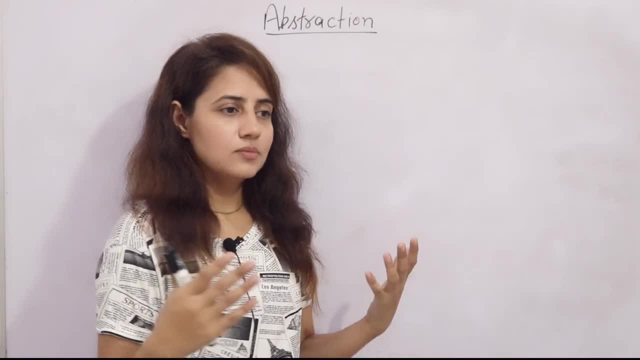 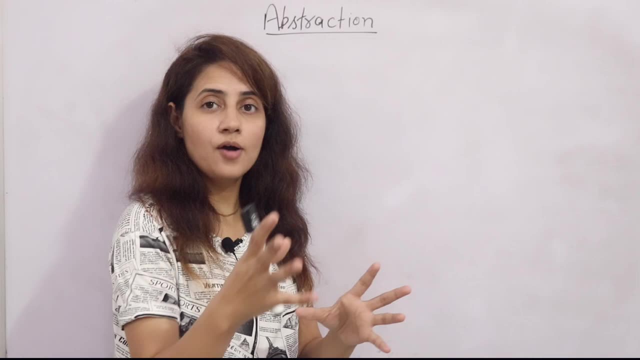 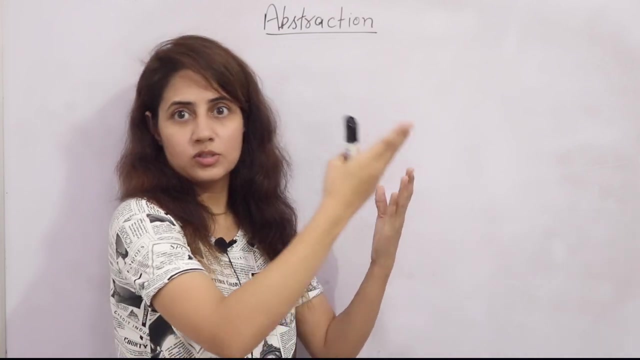 in this video. Fine, See, now I don't know, maybe you are watching this video on your laptop or on your mobile phone right Now. how you search for this video: You just open, maybe, the YouTube. then you search like maybe what is abstraction in Python? and there are. 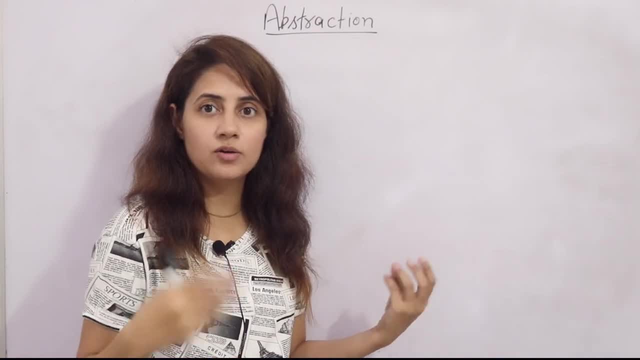 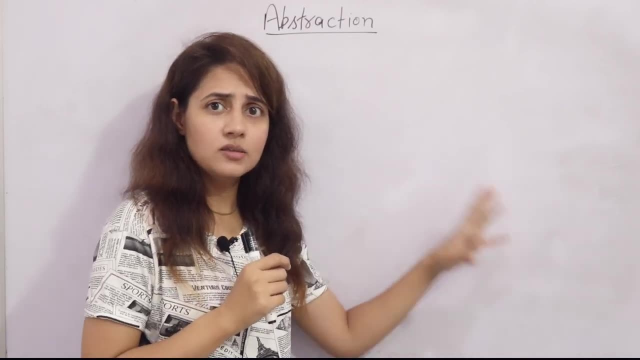 many videos in front of you. just click on one video and that video will be put on the on your screen, right? that is all you know, but you don't know what is going on behind the scene, how we are going to make you know, how we are going to a how. 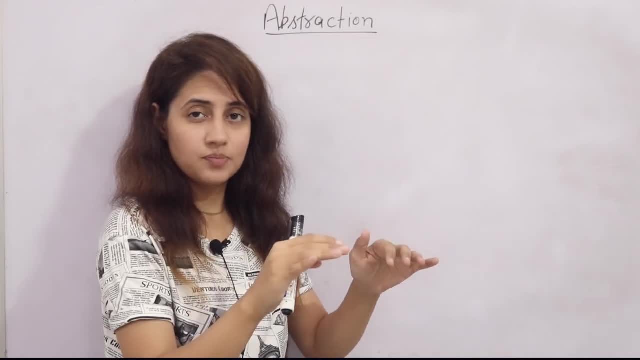 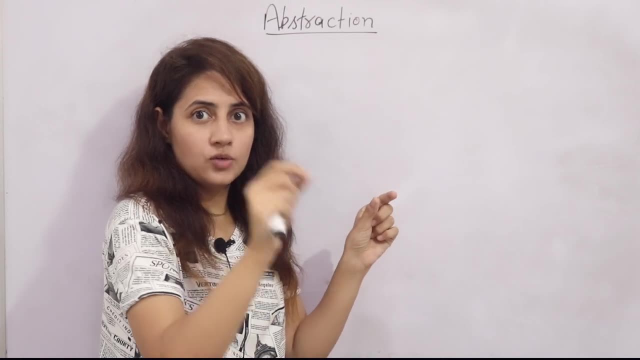 you are able to type like the alphabets, like and how. these alphabets have to be shown on your screen, on the search bar, like: what is WHAT, what is abstraction. you are typing with a keyboard or your keypad and these alphabets are shown in. 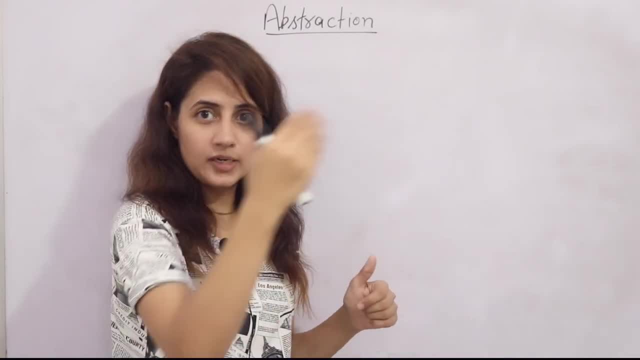 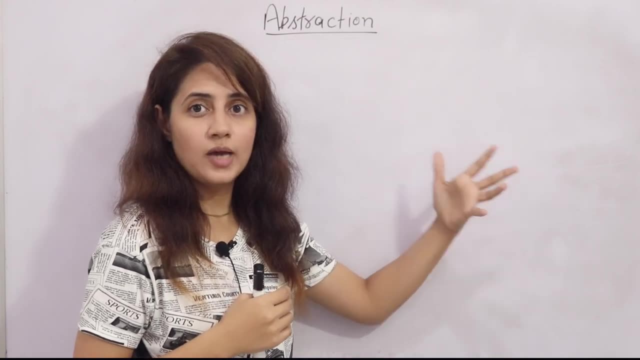 the search bar. when you click on the search, then you will get the. you're getting the results of these videos, right, abstraction videos. now, you don't know how this is going to be happening behind the scene, from where you are getting this video. obviously, when someone is uploading the video, then that 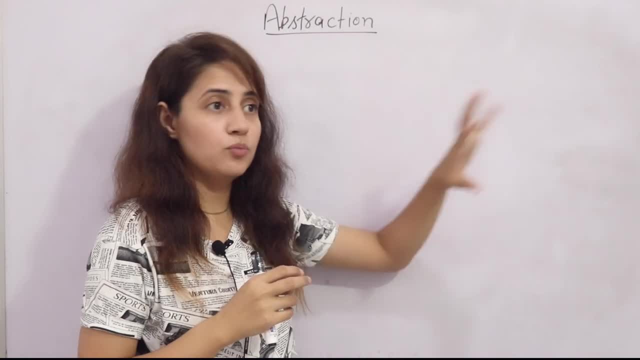 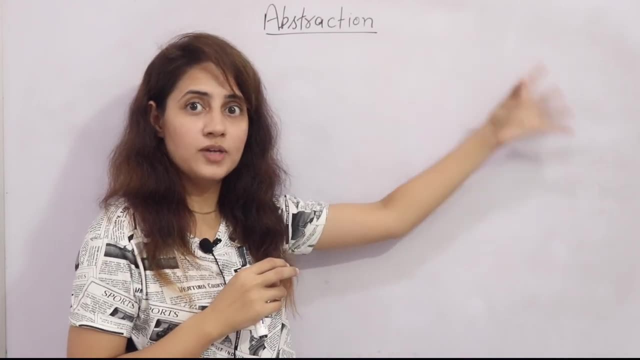 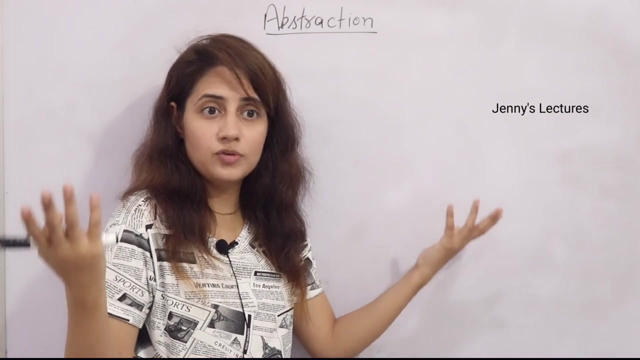 video would be stored somewhere in a database on server and from those servers you are connecting, you're going to connect your PC or your laptop or your mobile phone to that server and from that server you are fetching that video right and that is being displayed on your screen. you don't know, with the help of. 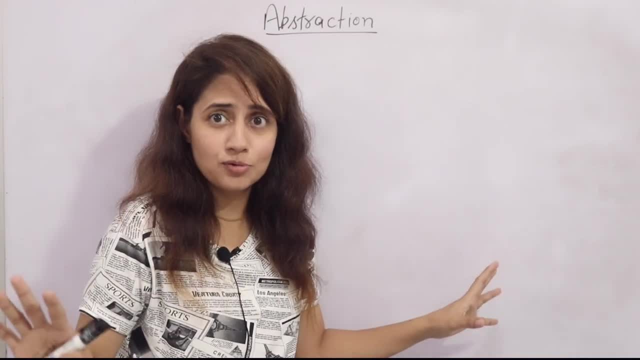 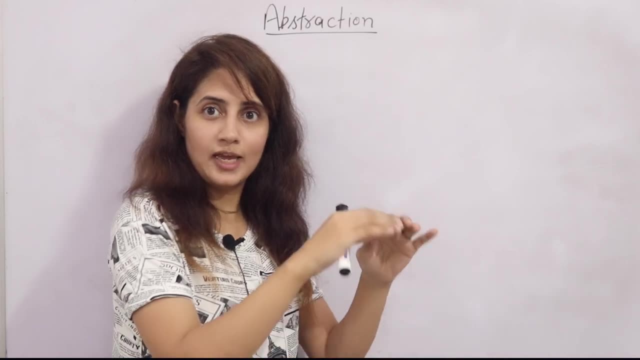 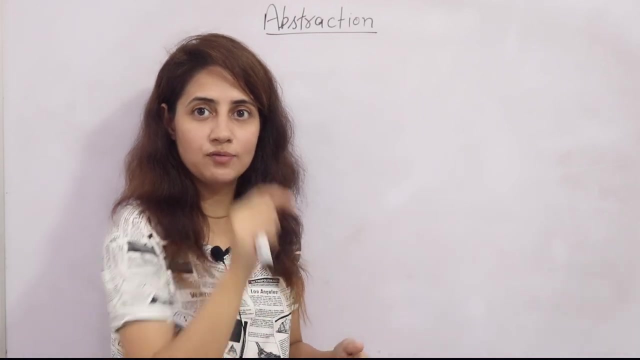 which protocol may be HTTP or FTP or I don't know any other protocol. right, you just know. you are just typing with the help of keypad or keyboard and just click on the search button and video is the search result are on your screen, and when you click on that video it would be just played on your screen. that's it, you. 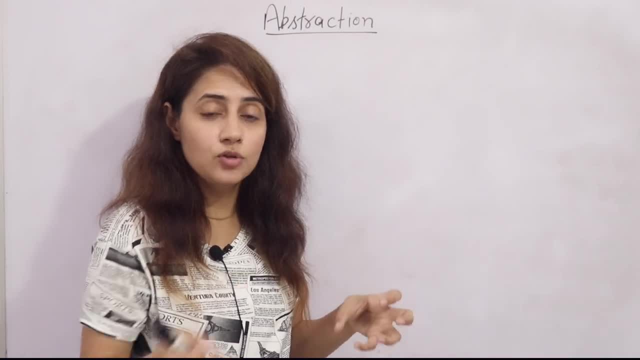 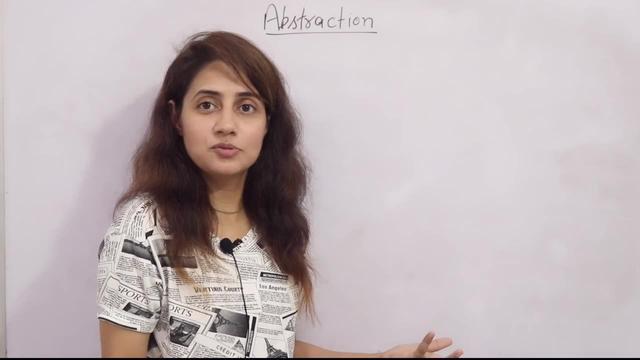 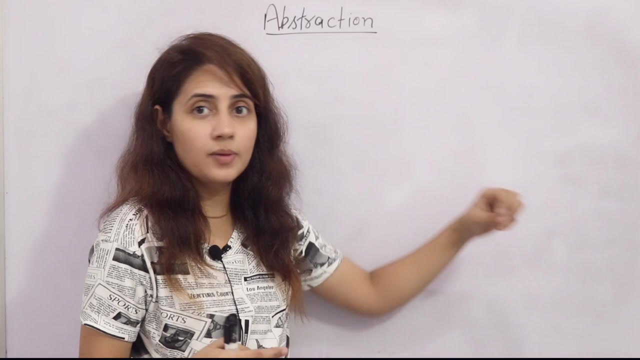 don't know the internal working are getting that video on your phone, on your pc, on your laptop, right. so that is what an abstraction. you're not able to see the internal implementation or internal details, or in the internal working or the behind the scene working. you just see the results. that's it and which actually matters to. 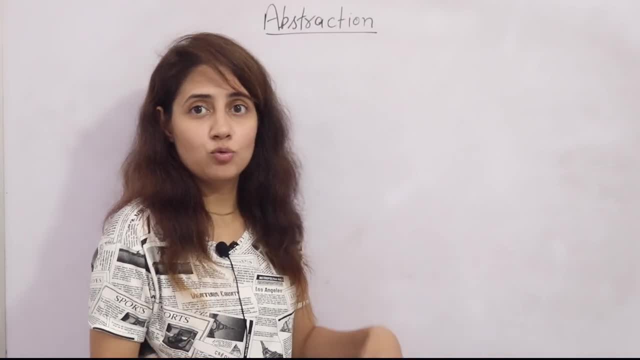 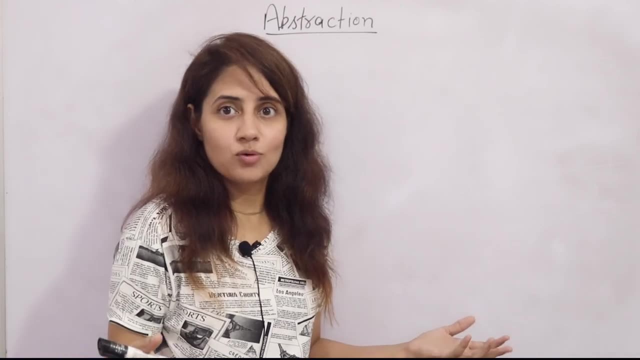 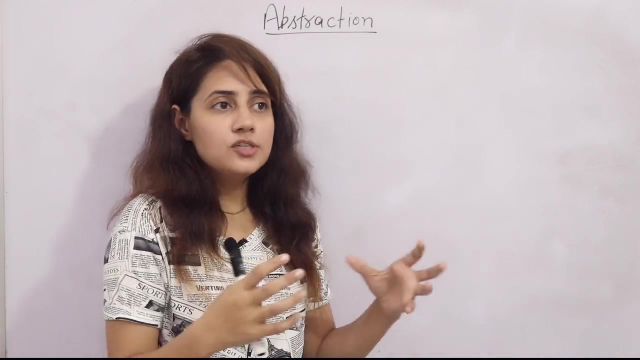 us the result only. we are not, you know, concerned about the internal working. maybe few of you are concerned about that thing, but many of us are not concerned about the how this is going to be working. we just concerned about the results. that's it, abstraction. in a similar way, just show the. 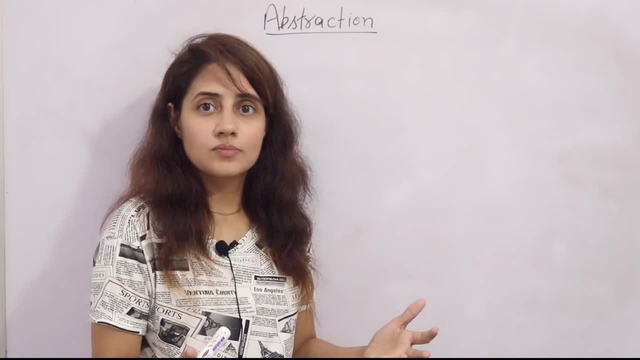 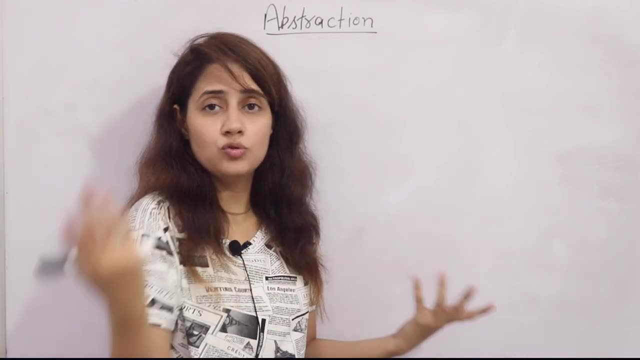 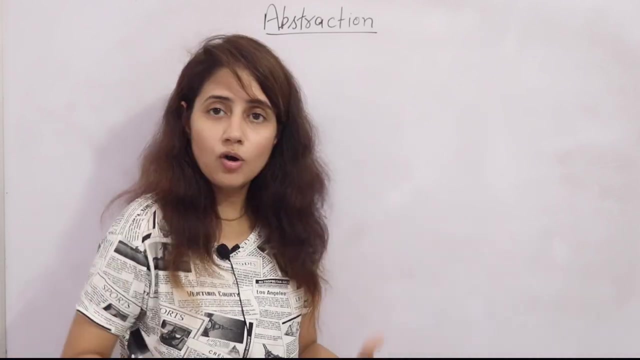 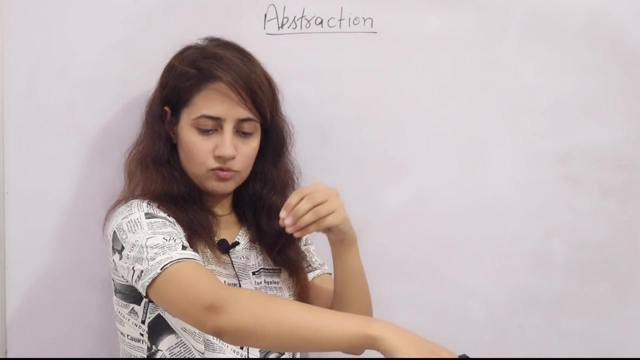 functionalities, anything holds hiding the internal detail or the implementation detail that are not, you can say, necessary to know to the user. simply, that is abstraction. everywhere we see abstraction, like we are example of abstraction, like our skin. this layer is an abstraction under the skin we have like 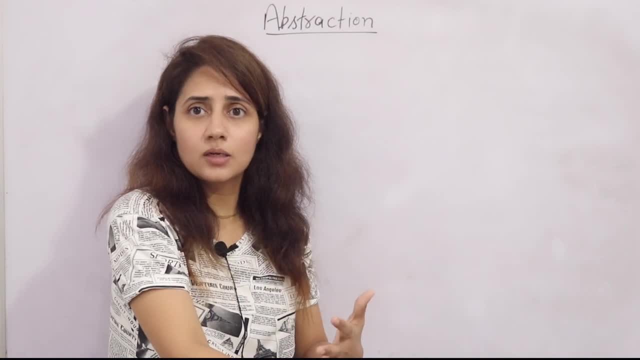 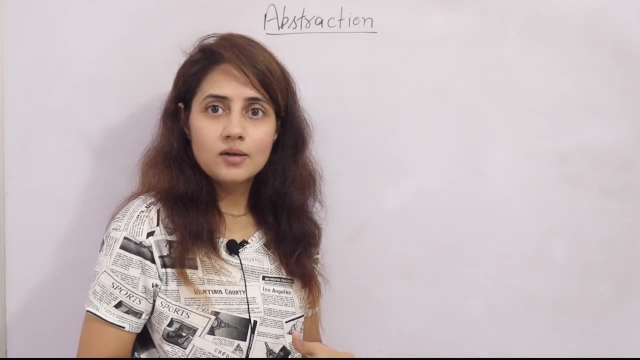 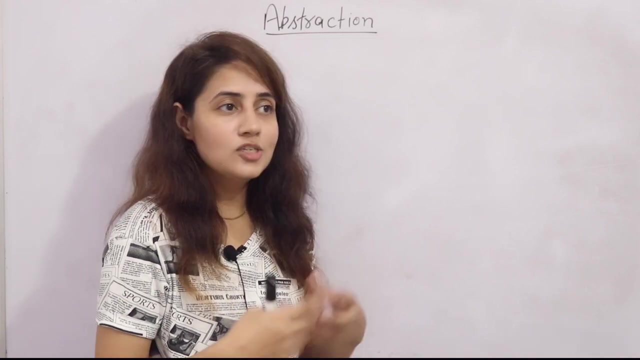 vein, how the blood is going to flow, the muscles and everything. we don't know anything. the lungs are working, how the lungs are working, how the heart is working, and we don't know anything, right? so the skin is a layer of abstraction for us. the internal detail is hidden. we just know the 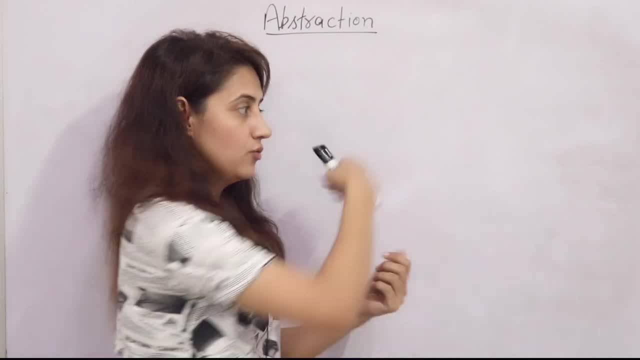 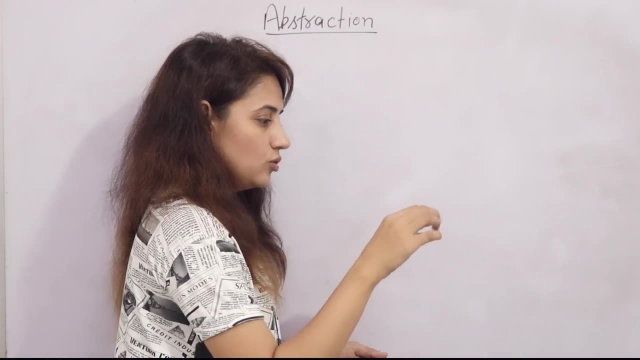 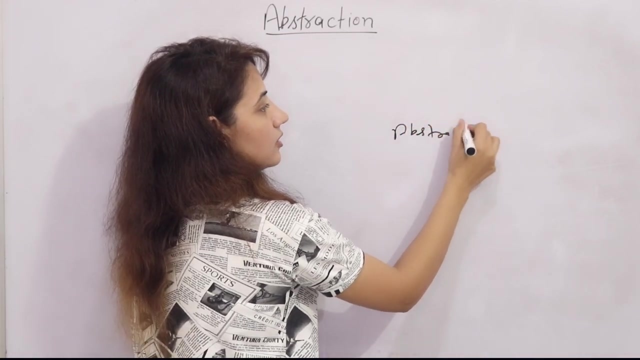 functionality is what a person can do, what we can do: we can see, we can write, we can walk, we can sleep, we can eat, but how? like how we are going to. you know, hold that marker. maybe when i'm holding this marker i'm writing something like this thing, then some signal is passing through. 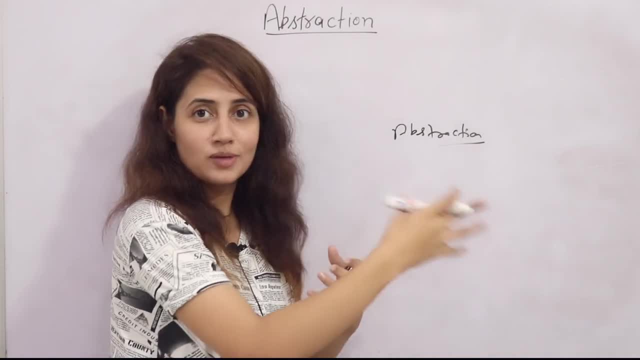 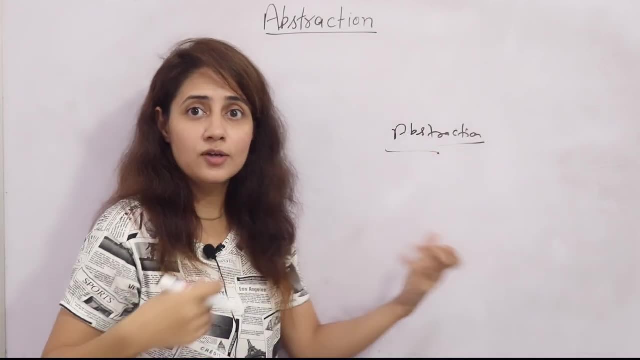 some veins or, i don't know, arteries to my brain and then my brain is going to instruct my hand or something like this. but that process, we don't know how this is going to happen. we just know the functionalities that we can write, we can walk right, we just sit back and think. 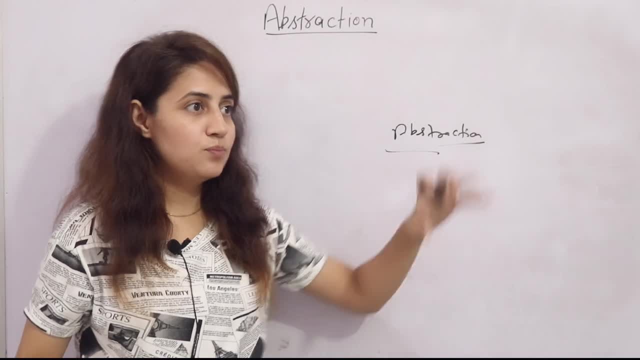 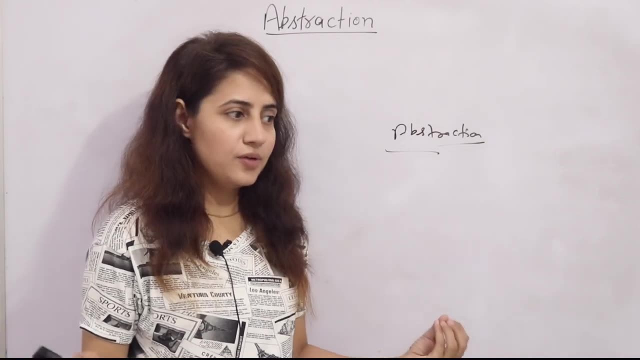 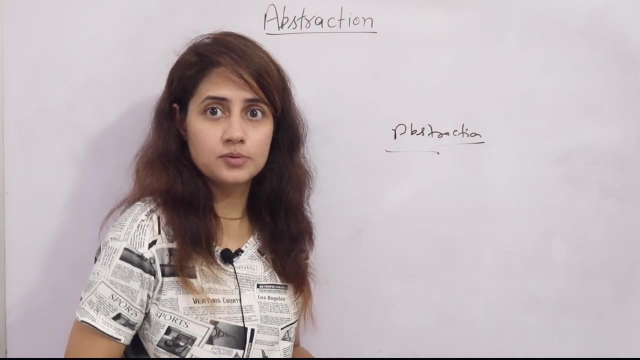 we can talk, we can like, eat, sleep, see or this kind of thing, right? so this is what abstraction. so everything in real world is also having some kind of obstruction and their level of obstruction, like higher level, higher level of obstruction, lower level of obstruction. like this levels of obstruction when you go to the. 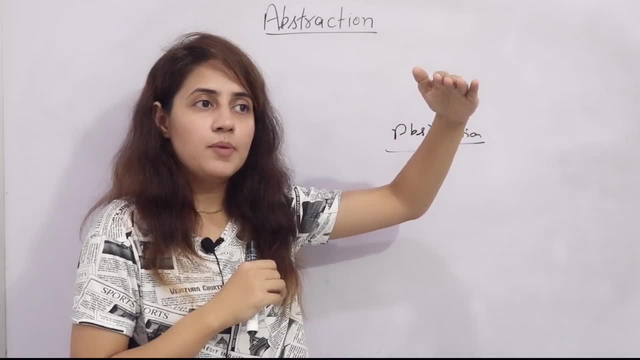 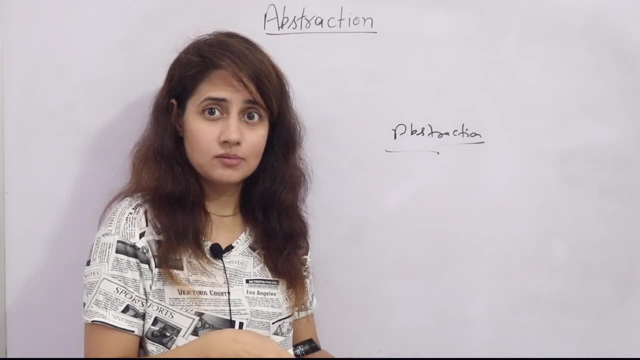 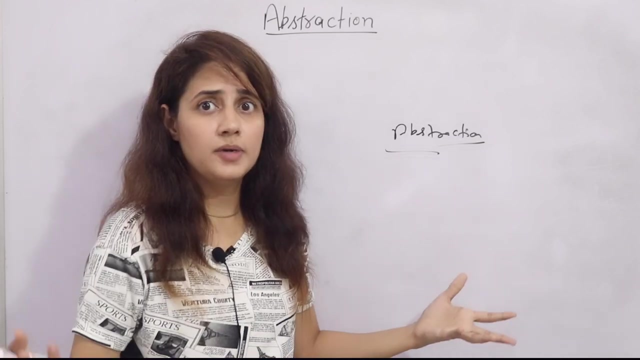 higher level of obstruction, then you concern about the larger piece of data, not the much detailed things, right like if I ask: just give me the highlights. if someone said just give me the highlights or just give me the minutes of the meeting or just give me the effects please, means I am just interested in an 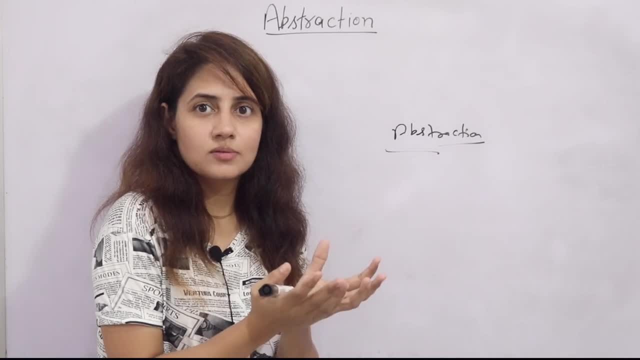 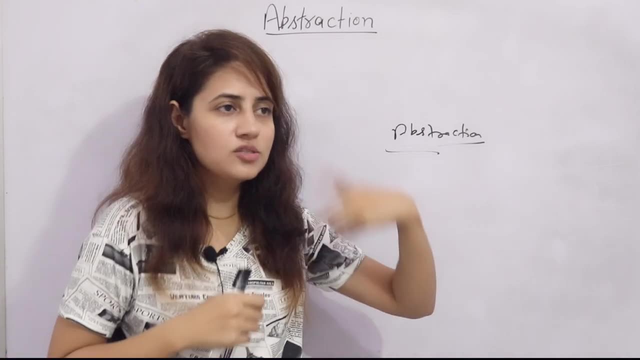 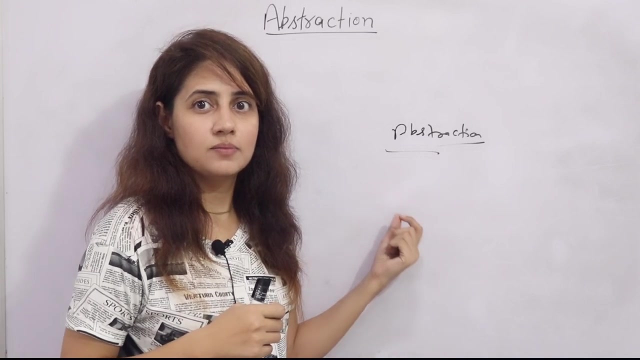 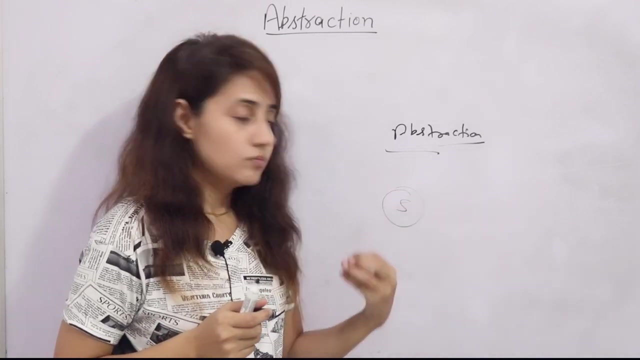 abstraction. these are the subtraction and abstracted way of information. I'm not asking for the detailed information, just the highlights, just the effects, just the minutes of meetings. maybe the meeting is for one hour, but there are five topics, mainly topics that has been discussed in that meeting. i just, i just want to, you know, i just want to ask those five topics. 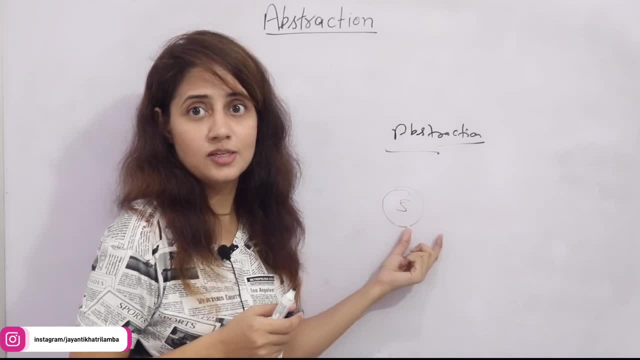 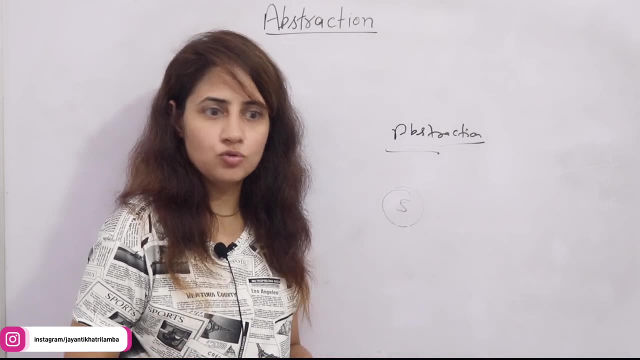 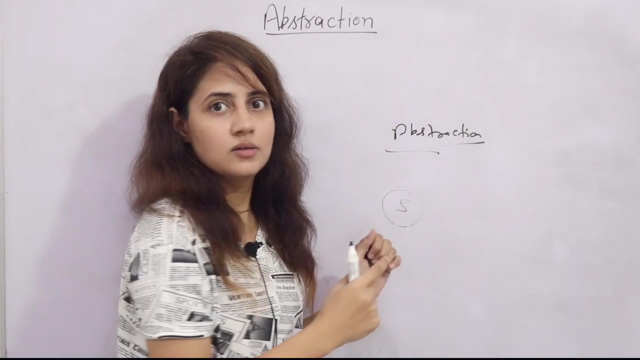 not what has been discussed under these topics in that one hour session. just give me those five points, that's it. so this is what abstraction you are asking for abstractions. if you have seen the research paper, then at first in this search where we are having abstract, 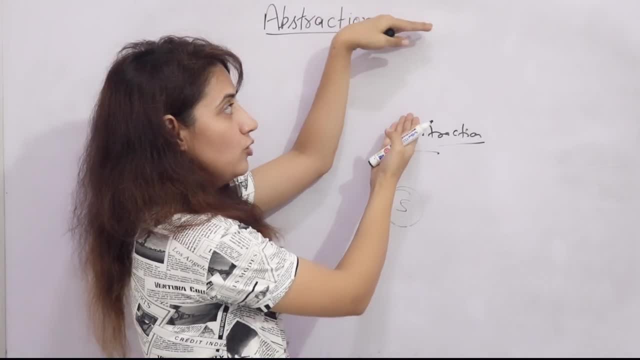 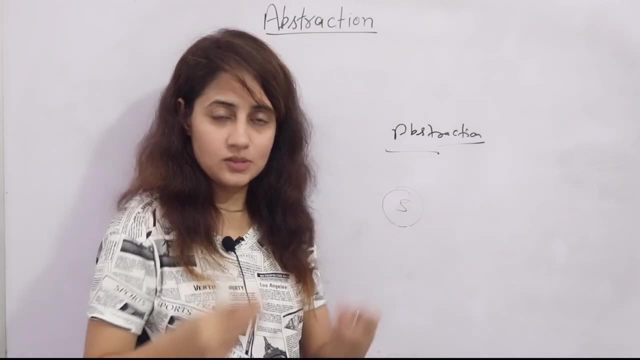 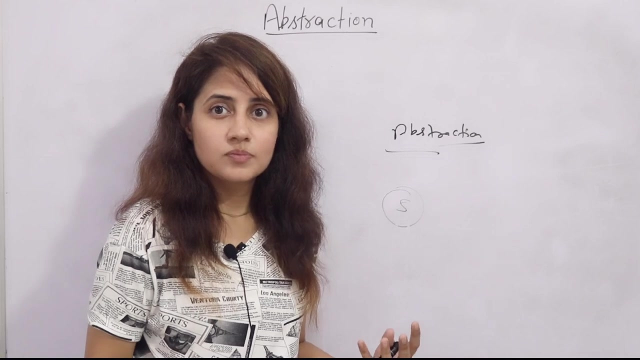 means that is going to tell you. that paragraph is going to tell you an abstraction like what is going to be in this research paper, just the main ideas or the main thing, what they are going to discuss in this research paper, what this research paper is all about. right, so that is abstraction. 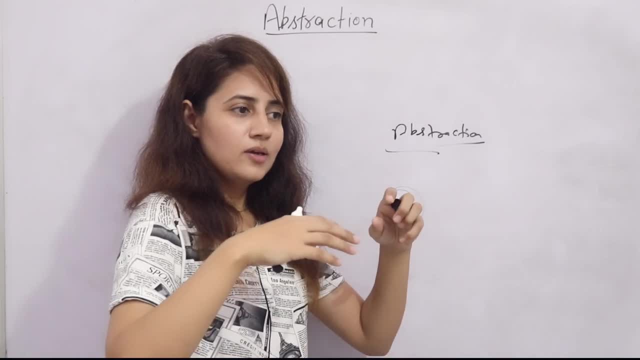 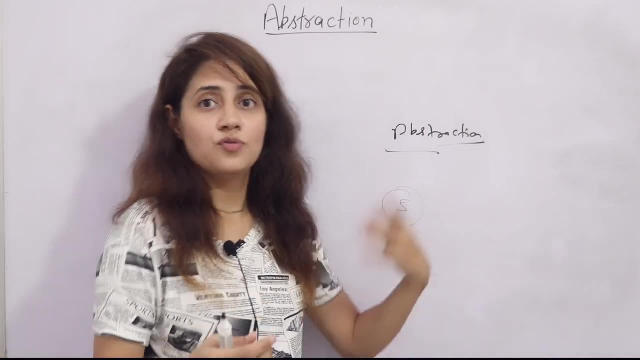 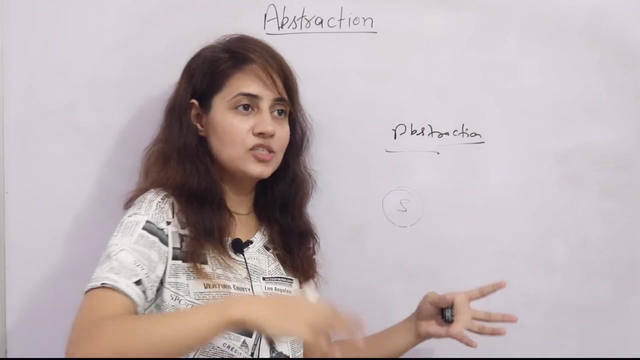 i hope you got this. so you, you, you, you are, you know, you get this type of you can say definition everywhere, like abstraction is a process of hiding the implementation detail from the user right, or the unnecessary detail from the user, or the extra detail from the user, the internal detail from the 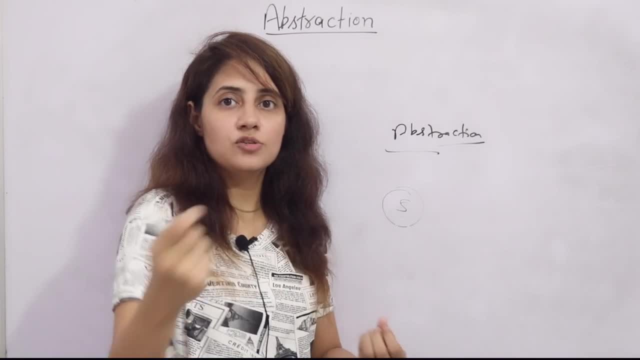 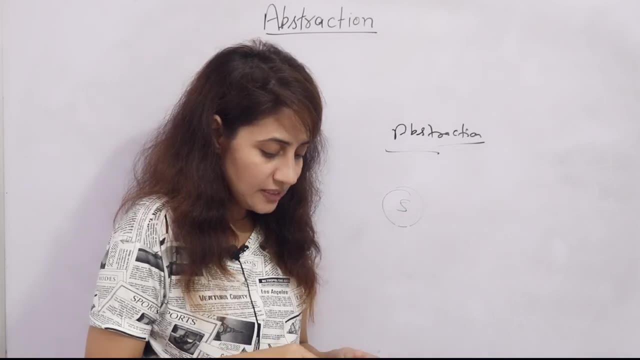 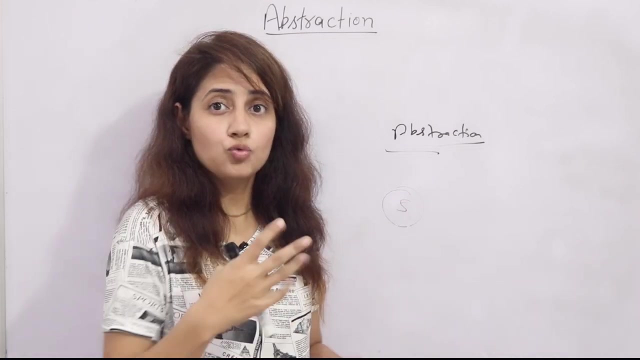 user, only showing the essential features to the user. that's it. that is abstraction right. that is one you can say definition of abstraction right. or we can say like. abstraction is also a general or generalization, or generalizing something to hide the complex logic. right, generalization means like. 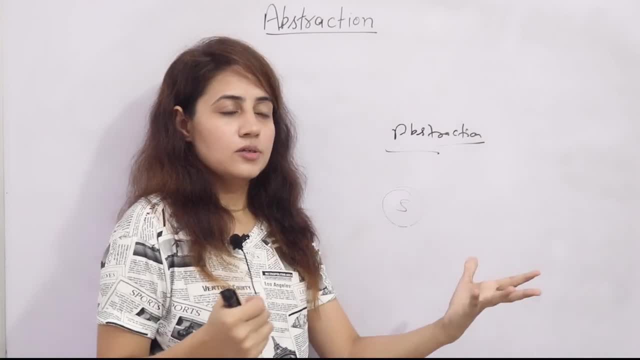 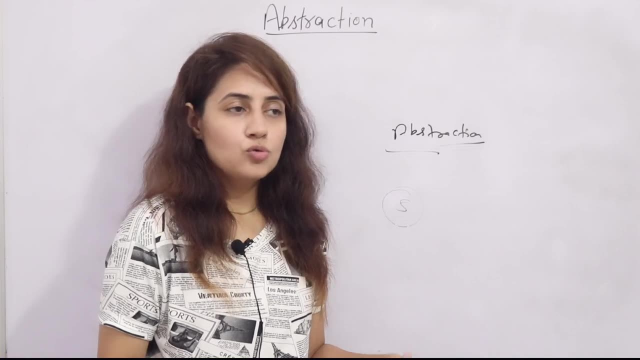 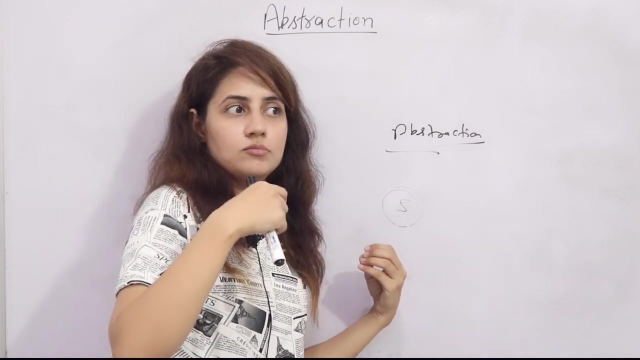 we a human being. we are able to eat or we are able to. we can sleep, we can eat. we have like two hands, two legs, so whether it's a male or a female, or a child or a- you can say a senior citizen, or maybe we can say it's a student or an employee, everyone can be a citizen or a student. 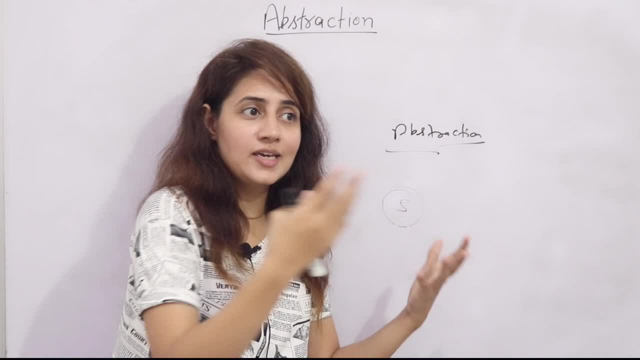 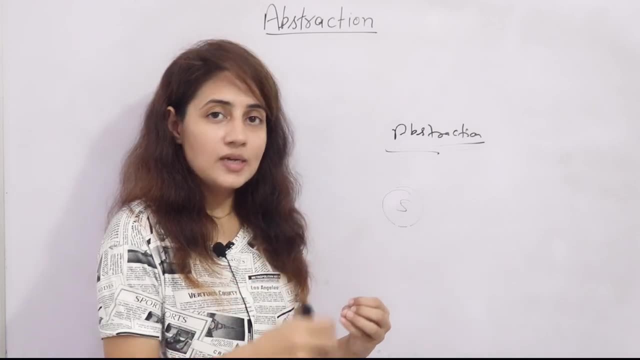 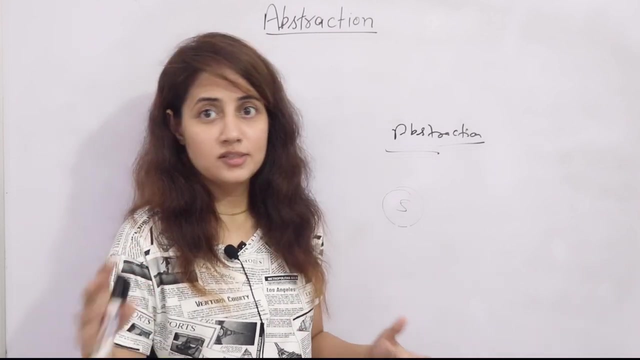 is having like obviously two hands, two legs, everyone can eat, everyone can sleep. so these are generalization or these are, you can say, generalized things that he or she can do. any male or female or child or senior citizen can do right. so in programming also, if you want to. 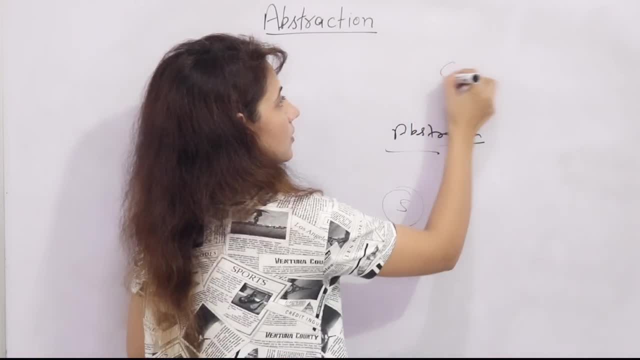 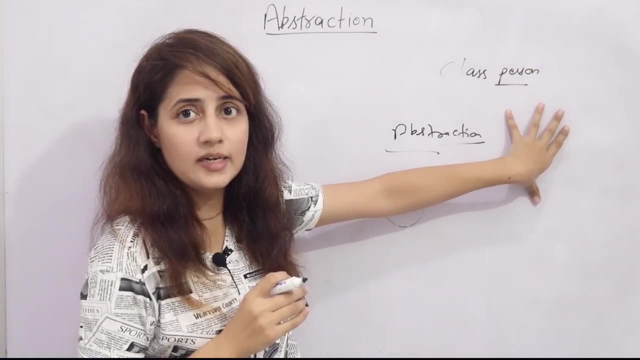 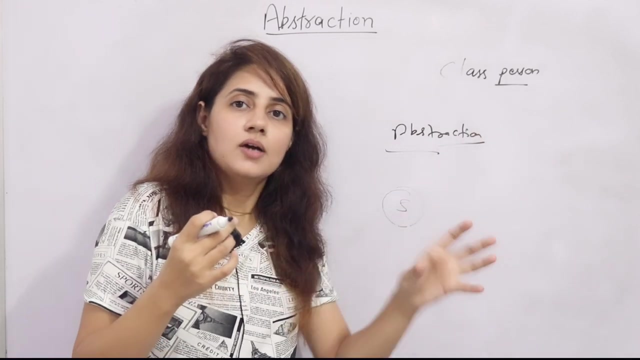 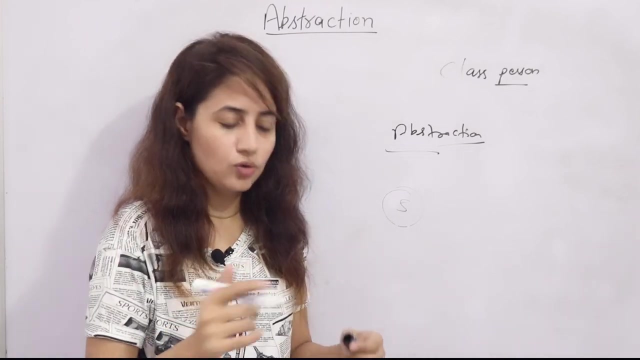 represent this kind of thing, then we can make a class person. and here, in this, we can abstraction. we can, you know, achieve abstraction with the help of abstract classes and abstract methods. right, what are upset classes and methods and how we are going to achieve abstraction? that we'll see in next video. but here, 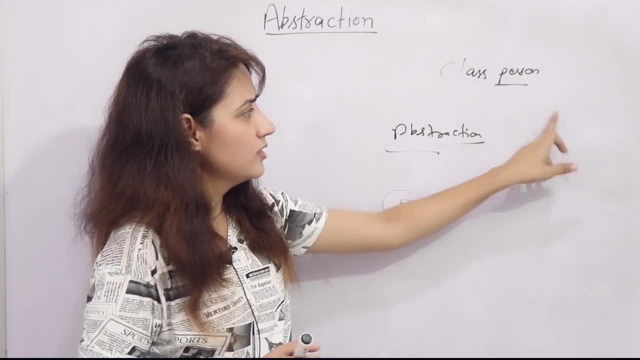 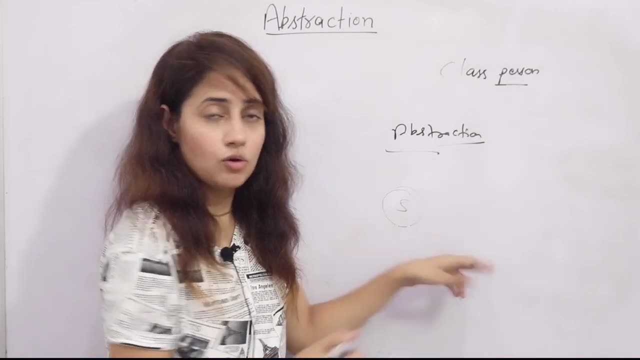 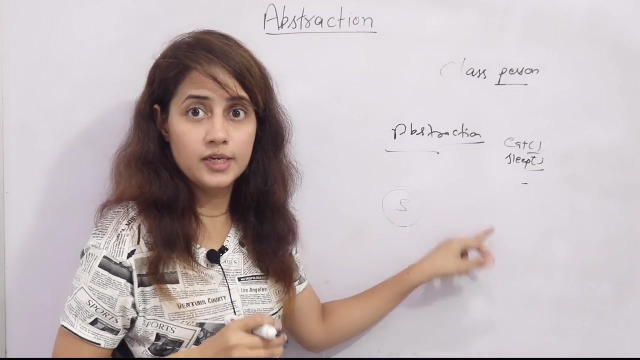 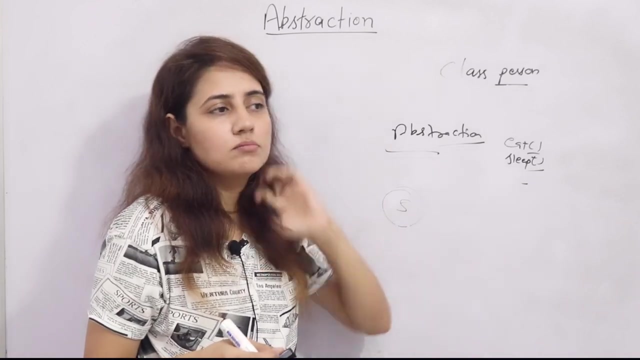 we can define like number of number of legs, number of eyes, number of hands, like this and every other class which is going to inherit this class, definitely, obviously. or like some functions like eat, sleep. we have these functions like eat and sleep, but maybe they have their own definition of these functions. eat, it is what maybe eating. 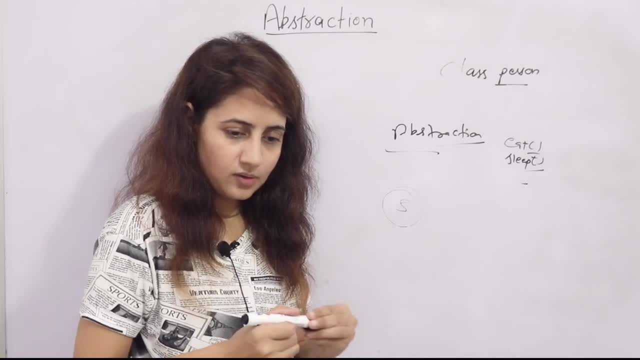 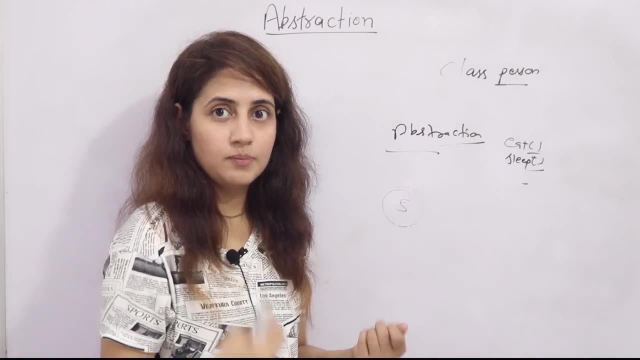 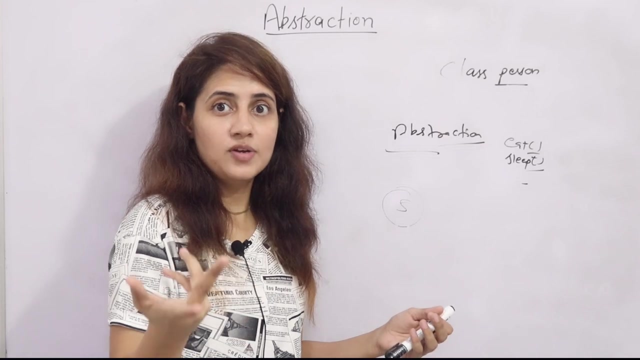 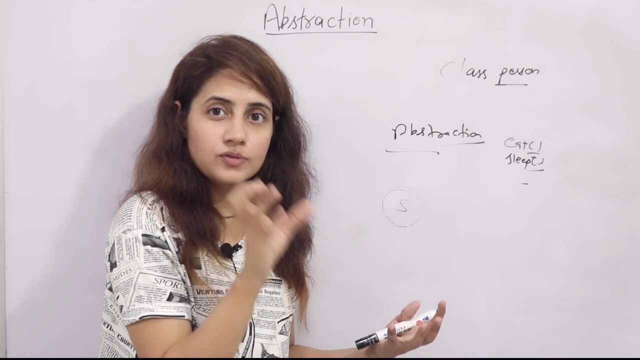 habit or eating process of every person is different. like I want to, I would like to eat with knives or that fork and spoons. maybe someone is interested in just eating with hands only. that is also fine. so everyone is having their own process of eating. but eat, that is for sure. that is for everything. that is a 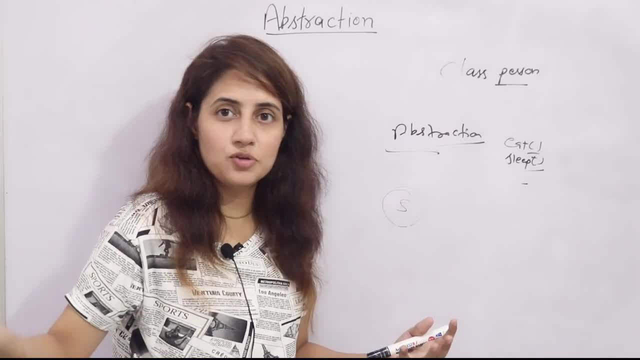 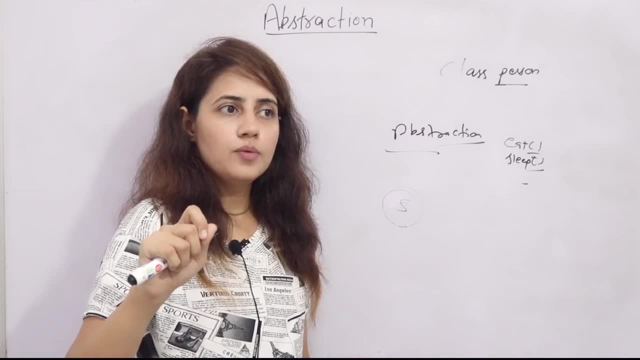 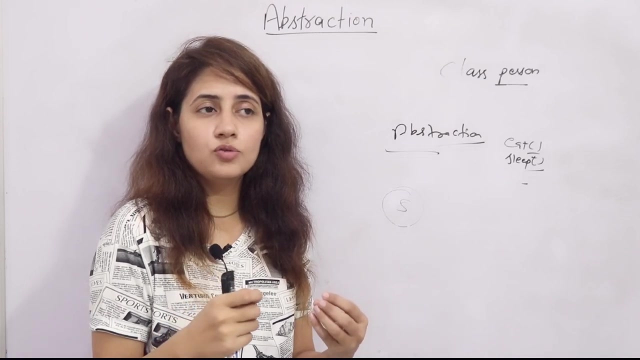 you can say generalized thing for every person or every human being, right like. let's take one more example: if you are going to make any app, develop any app, so every app is going to have some. you can say general features, like the brightness feature or the every app. 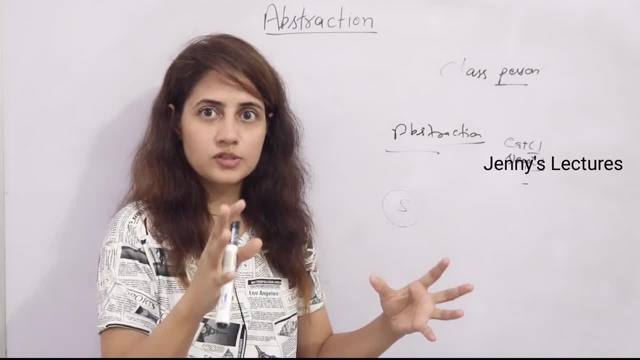 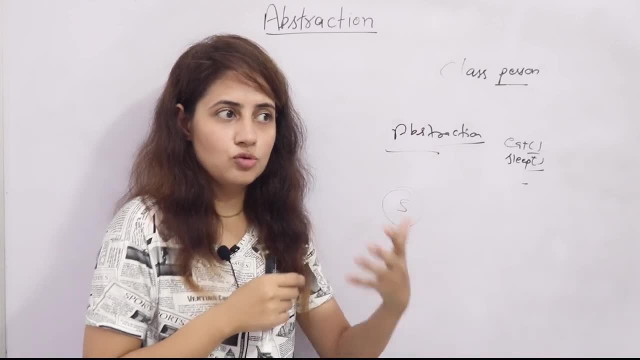 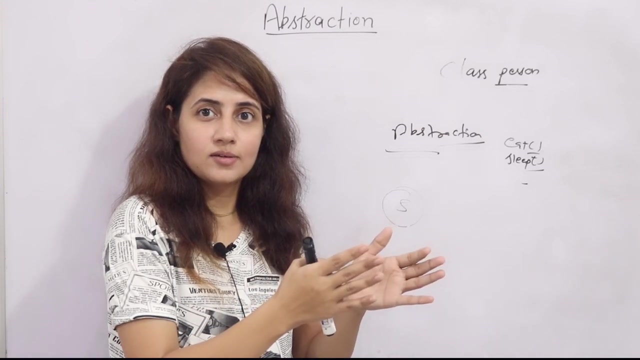 is going to send notification right. those features, every app, any app in your phone you have, you can know that the brightness feature or you can say that notification feature, right. so that is what generalized thing is. so if I'm going to make my app like for Jenny's lectures, obviously that also. 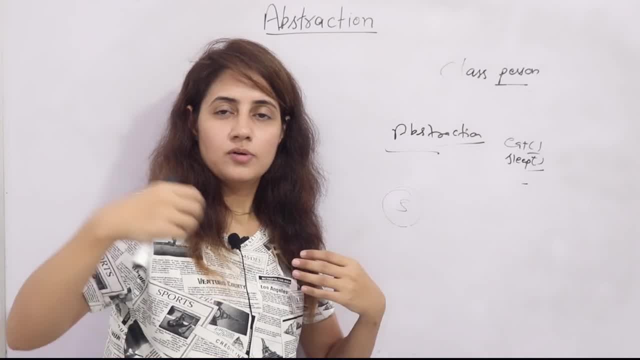 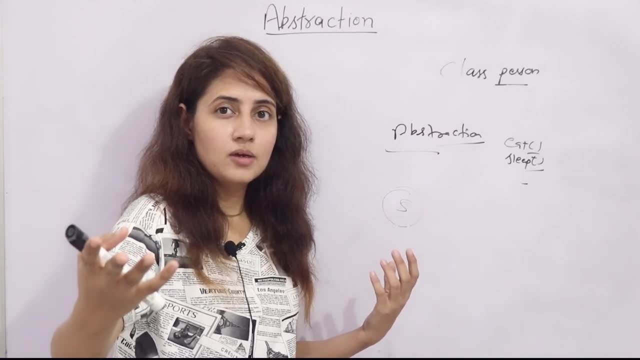 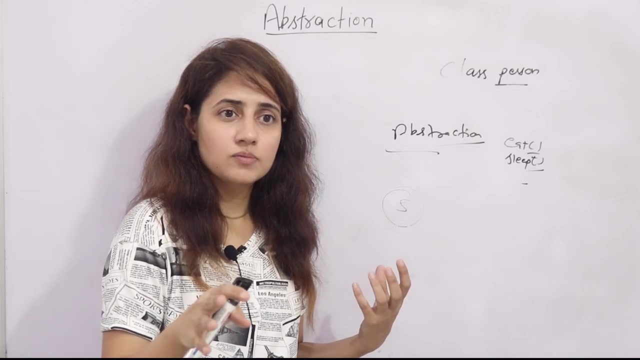 have that send notification feature, right. if you are developing any other app, maybe like related to any image, or you can say upgrade your image or edit image, these kind of things, like picasa and anything- those will also have that feature, that notification feature, send notification and all right. so 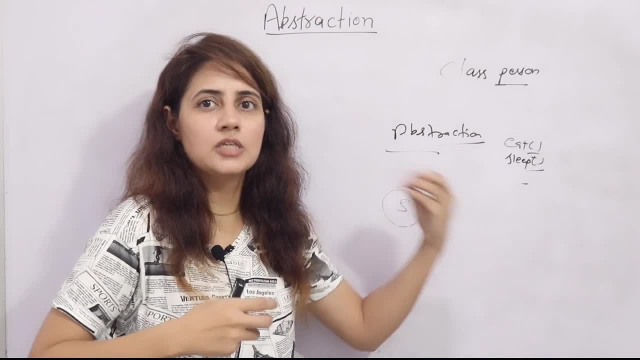 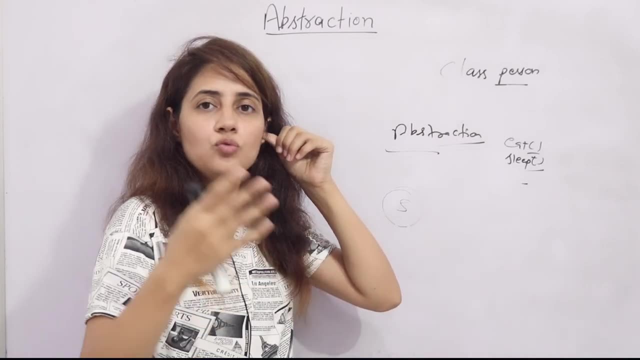 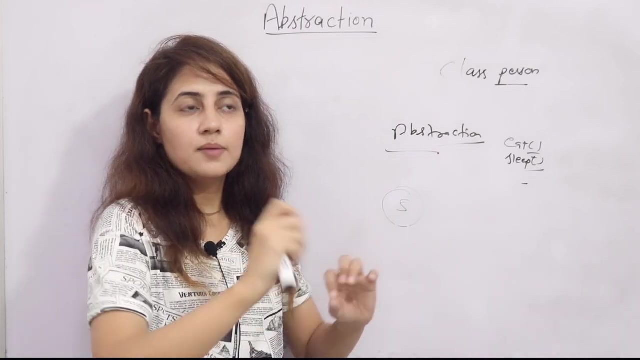 this is what we can achieve with the help of abstract classes, right, but how we are going to achieve that thing, that as shown in the next video, just though, which I use. so what is abstraction? we can also say in another term like it is generalizing things, or we can say abstraction as a process of generalizing in something. 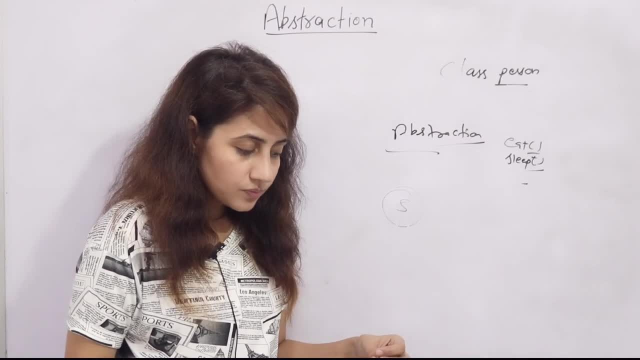 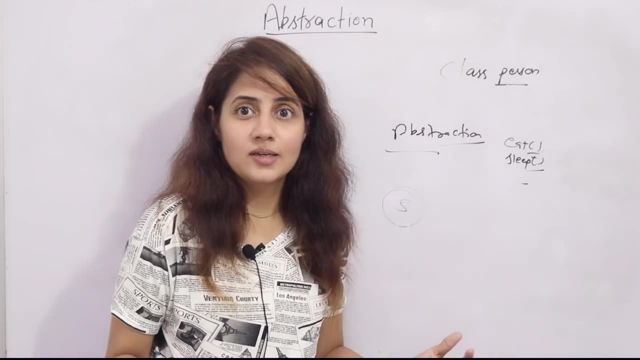 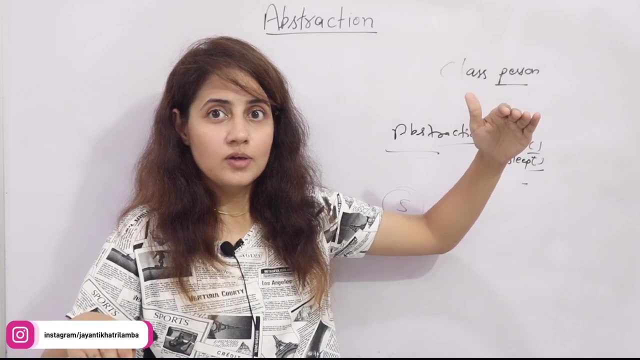 just to hide the complex details. now, how to hide those details? abstraction is just a thought process. it works at design level, design level, not at actual implementation level, that coding level. no, so you can say it's just a process of identifying which features are to be. 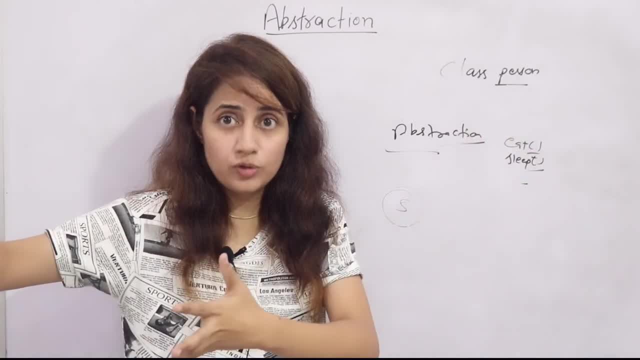 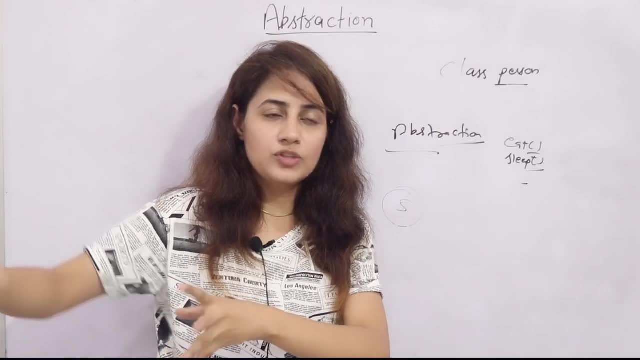 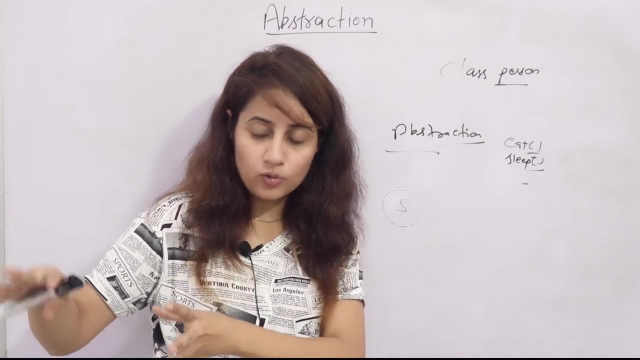 hidden from the user and which features are to be shown to the user. you just have to identify. but actual, how we are going to hide, that is a different thing. with the help of encapsulation, we'll do that, that, that thing, right. so actual you are. when you are going to hide, that is a different. 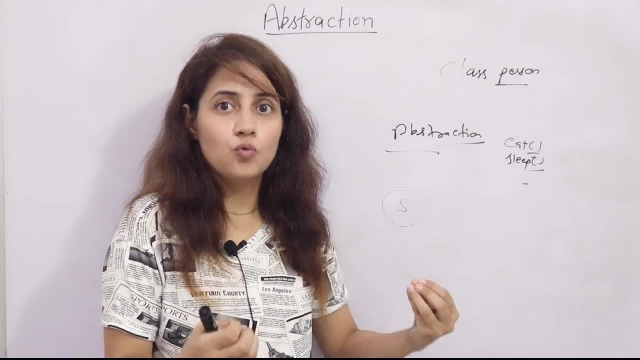 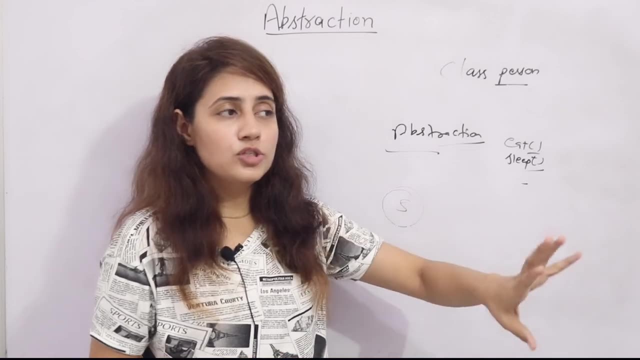 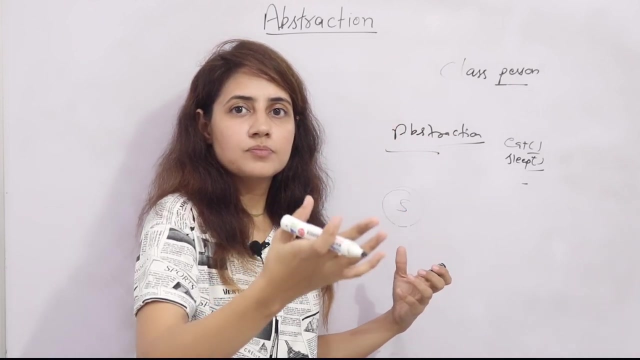 concept, concept, but in abstraction, you just have to identify what you need to hide from the user and what you need to show to the user, right, if you are working on a project or any app or something like this and you have to add, like student name and data roll number, right? so this is some kind. 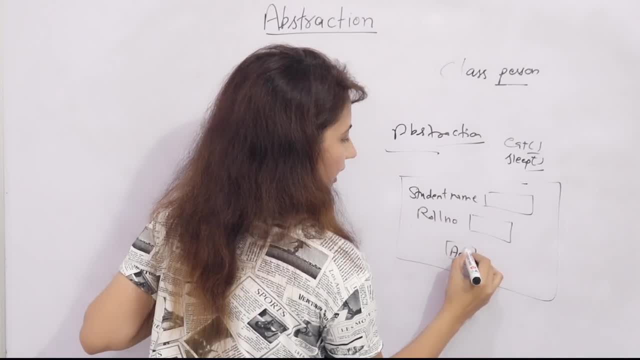 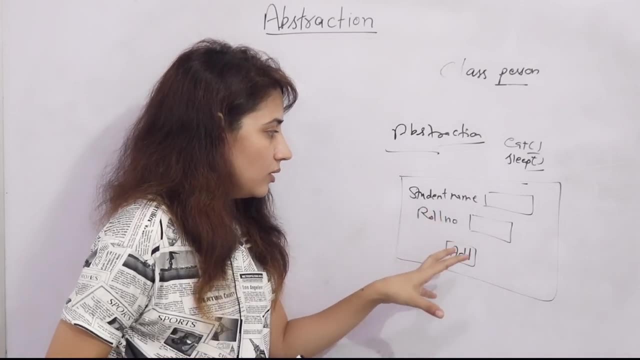 of introduction. the face would be shown like student name. like I am having, I'm just working on any project like maybe student management system, so I have to add student detail. so you can just show student name, it would be entered. all I'm going to enter, I just have to. 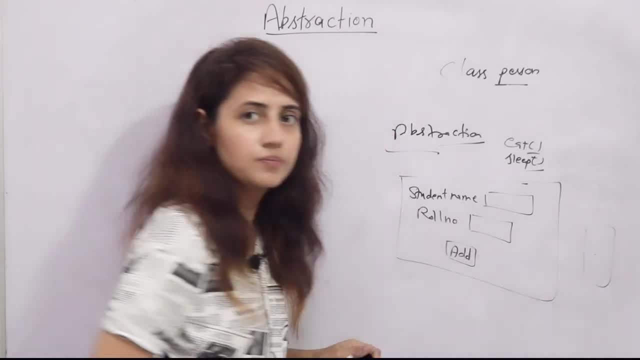 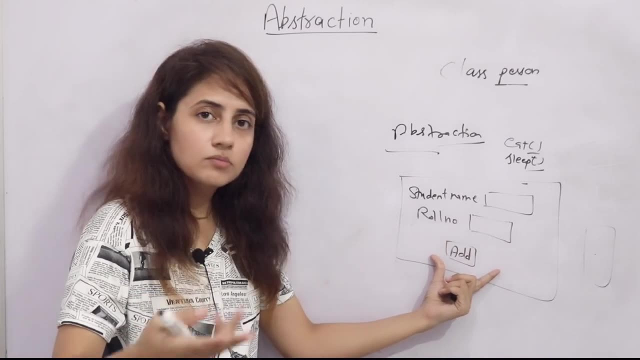 click on the add button and in the database that student would be added right now. that's it. this is the interface that would be shown to the student or to me, or the user who is going to be shown to the student or to me, or the user who is going to be shown to the user who is going. 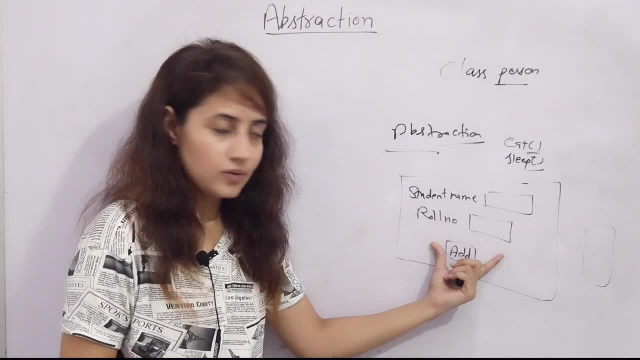 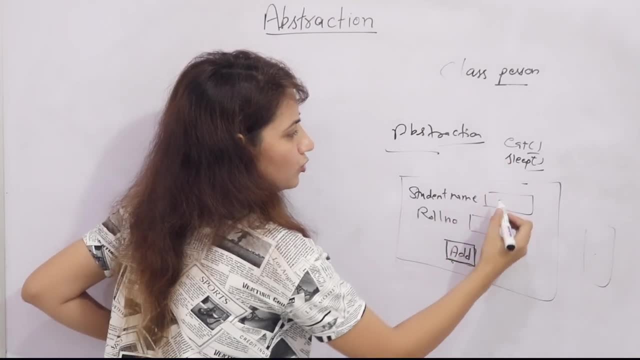 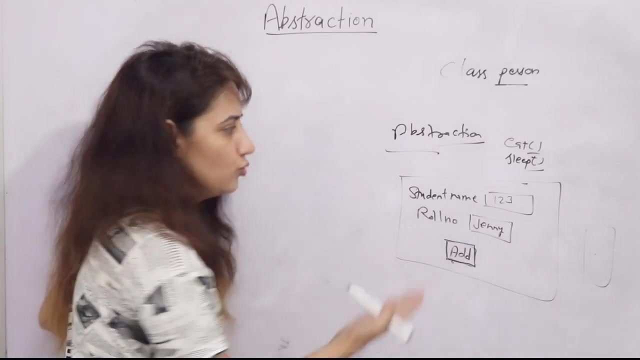 to use the student management system, this project, right now. add means obviously when you are going to click on add, then we will check. like maybe in student name you will enter one, two, three. in roll number you i am going to enter, enter jenny. so this is not valid student name should be jenny. 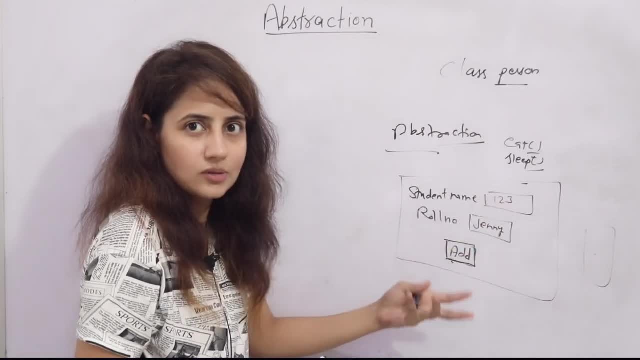 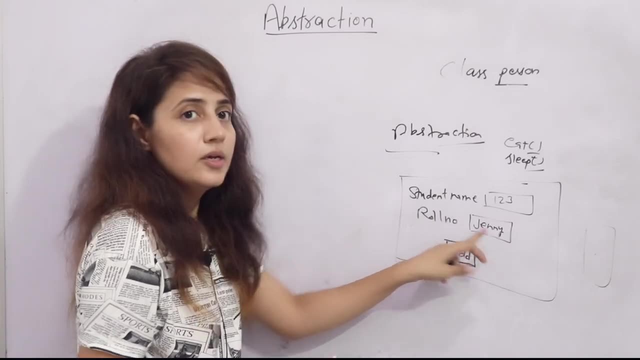 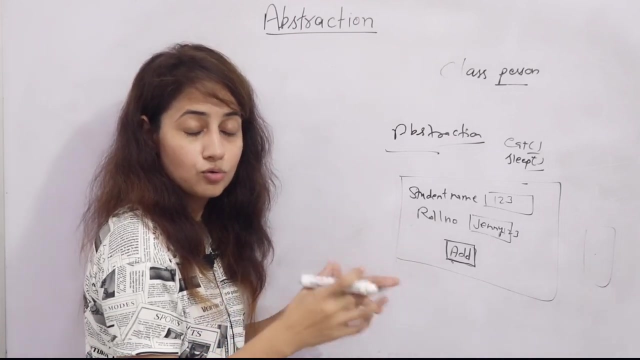 and roll number should be one, two, three or this kind of thing, right? obviously anyone can tell that this is invalid. roll number cannot be like jenny. it can be like jenny one, two, three. it can be combination of like alphabet and those digits, but only letters or only alphabet. that is not. 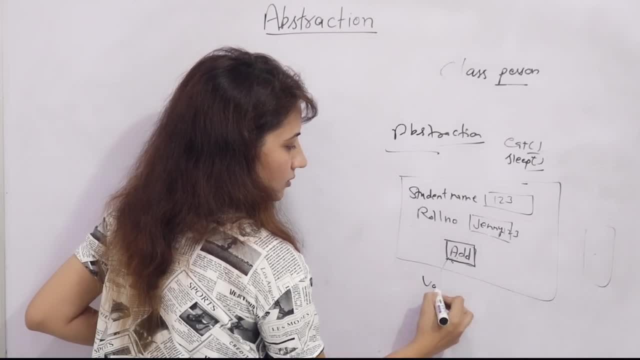 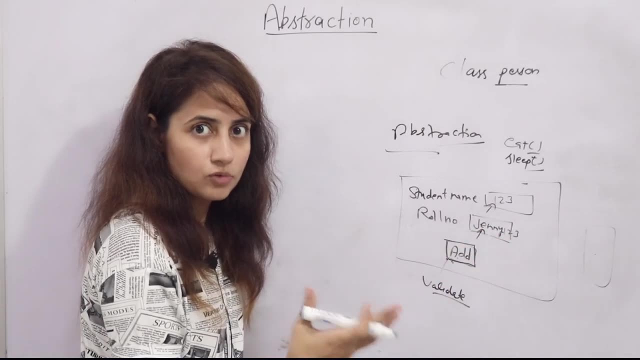 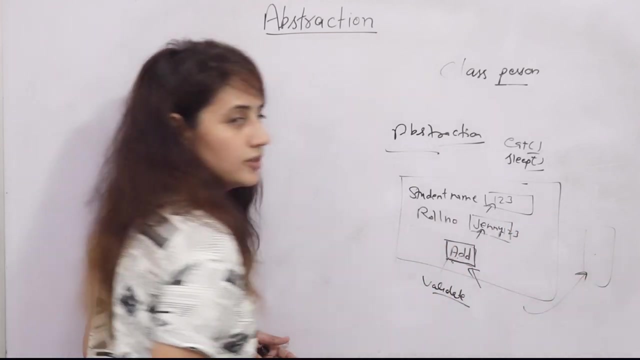 allowed in roll number right. so obviously, when you are going to add, then validate, or you have to check if the entry is correct or not according to the rules, are or not right and then create a database object and then add to this database. but this validate and create a db object. that would be. 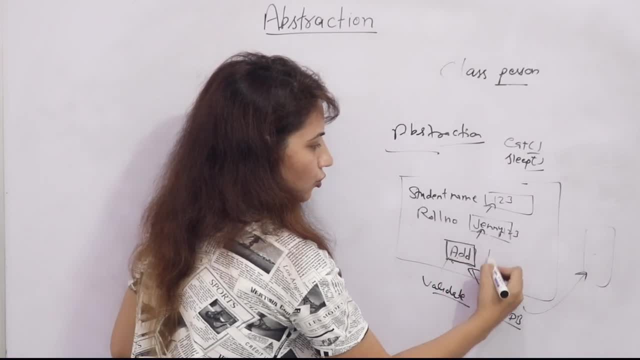 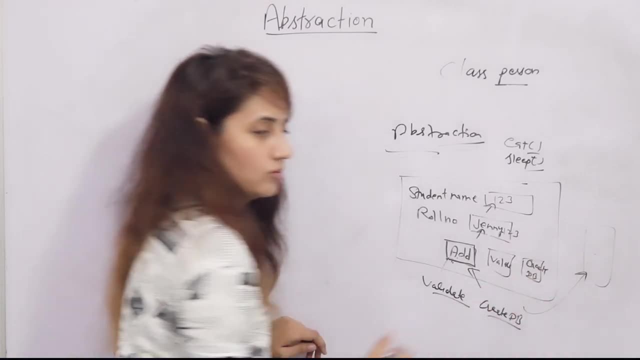 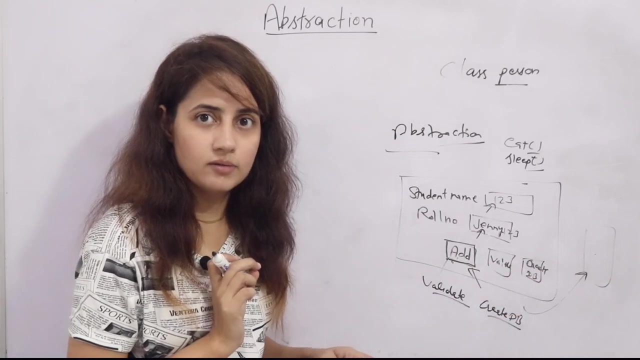 obviously hidden from the user right. we are not going to show in the interface like validate and like create a db connection, right, and you have to enter, you have to click on validate as well as well as create db and then you'll have to add and you have to click on the set then that student. 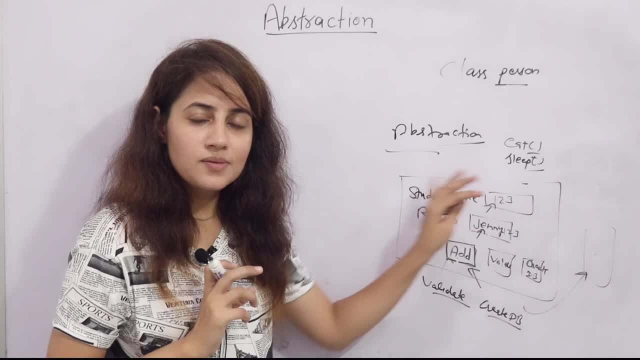 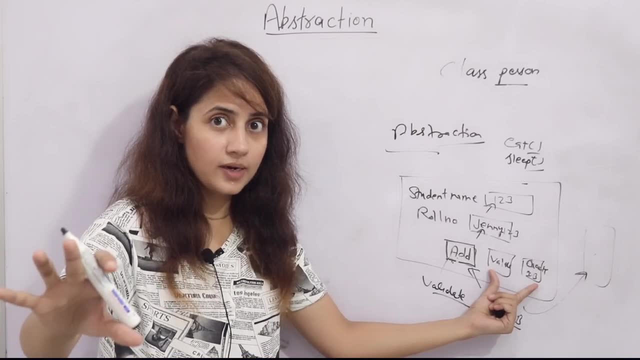 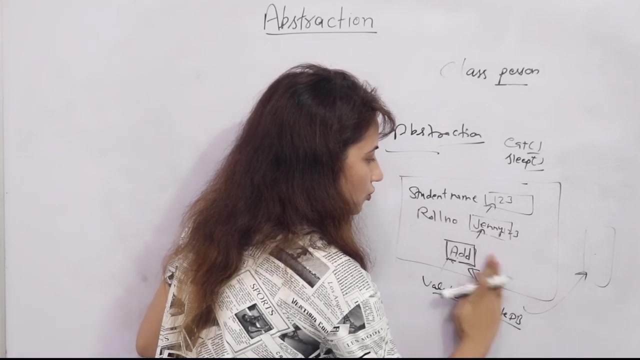 would be added to this. no, just a simple interface would be shown to the user. because these are extra details, these are internal details, so these should be hidden from the user, right? we have identified these two functions should be hidden from the user, right? so these are hidden from the user. 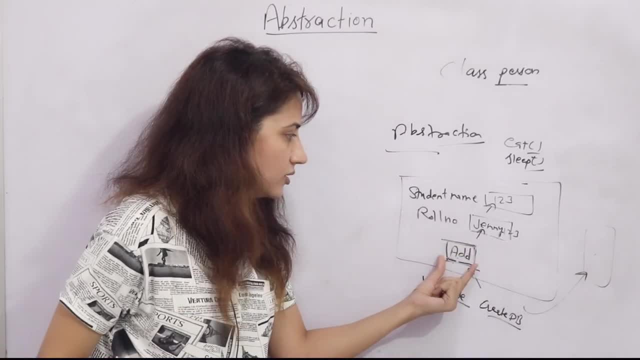 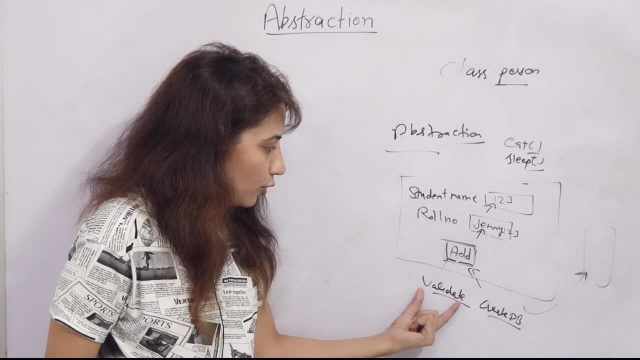 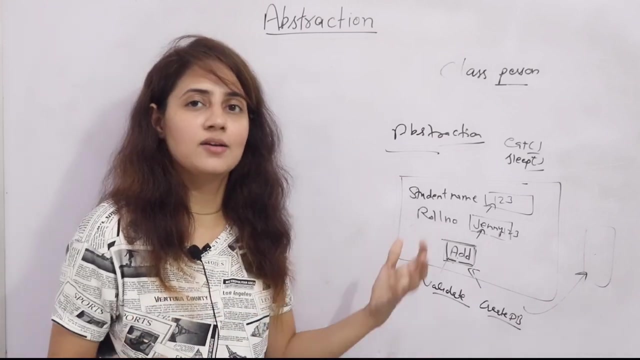 and only the essential information to be shown to the user is just the add button, right. so this is what abstraction right now, how we are going to hide these things that comes under encapsulation. we have some like those public private access specifier. with help of those, we can.